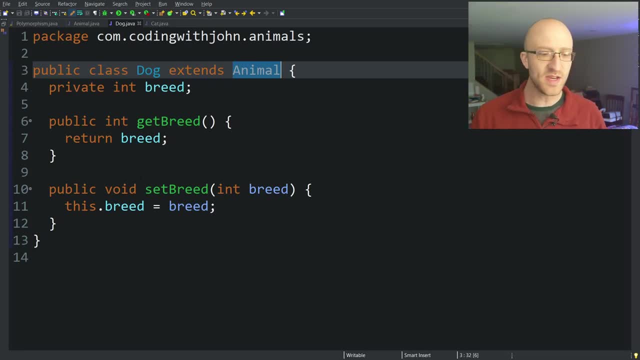 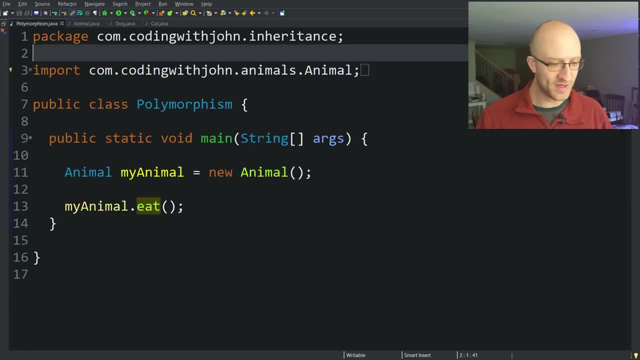 all the fields and methods of that parent class. So what does that mean here? This eat method, that's in the animal class. I don't have it written in the dog class. But because dog extends animal, I can go back to my main method And I can create a dog. myDog equals new dog And I can. 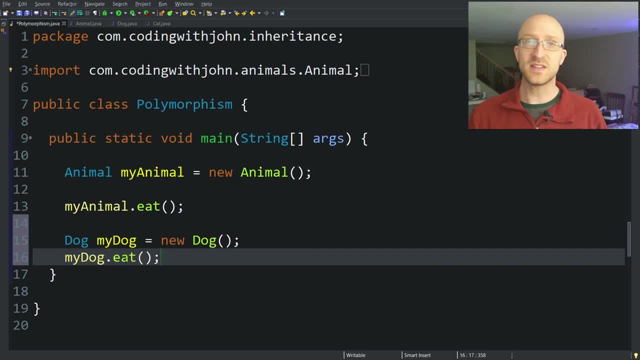 call myDogeat, You can see that that method is available, even though we don't explicitly have an eat method in our dog class. So I can go back to my main method and I can create a dog. myDog equals our dog class And we can go ahead and run this program as well And we'll see our animal eat and 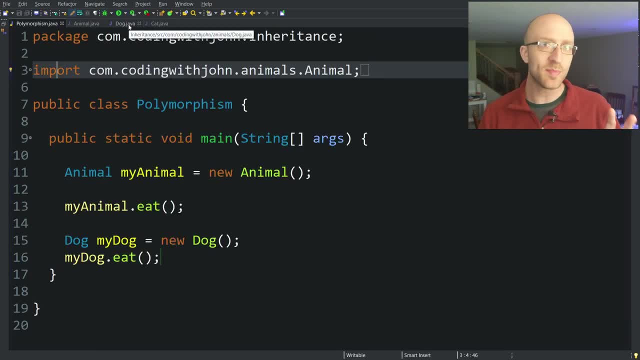 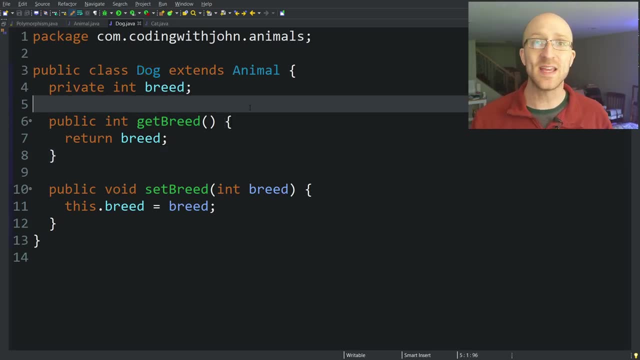 our dog eat And they both print out munch. But now here's where polymorphism comes in. Even though this dog class automatically gets that eat method and I don't have to do anything, by default it has the exact same behavior. In other words, if I don't do anything, my dog is going to eat in. 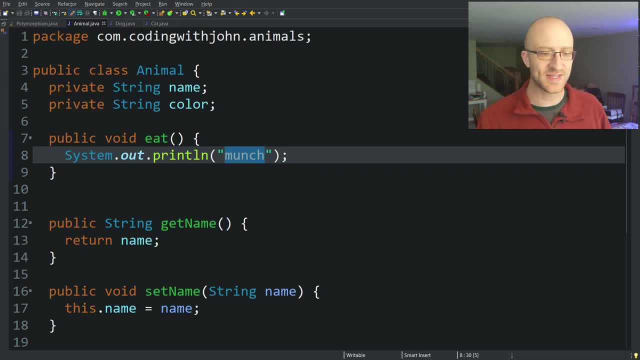 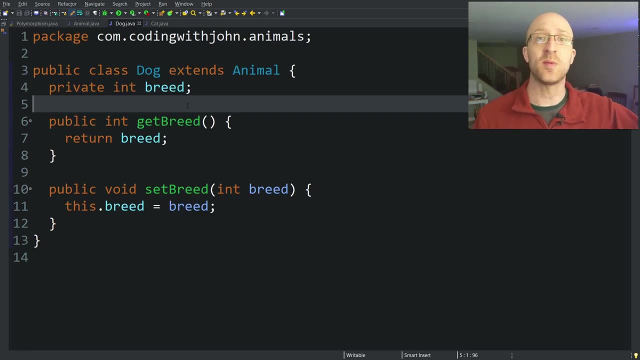 exactly the same way as any other animal. It just prints out munch because I didn't specify anything else in my dog class. But what I can do here in this dog class is override that eat method from the parent animal class And if you want to override a parent method you have to implement. 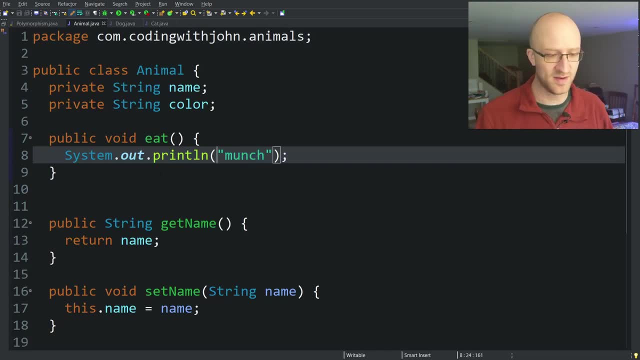 the exact same method signature as that parent method. So we can see the method signature here is public: void- eat. It's a public method. It doesn't have a return type, so it's void. The method name is eat and it doesn't take in any parameters. So over in our dog class, we want. 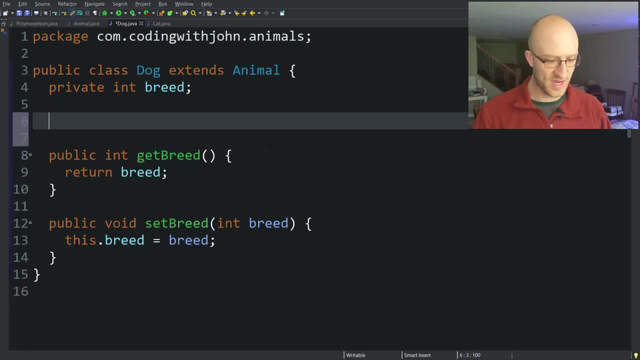 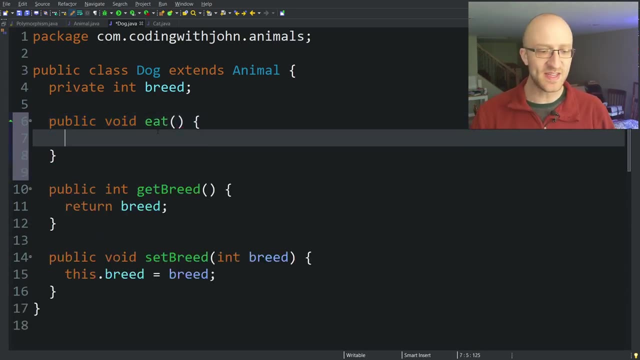 to implement the exact same method, signature to override it. So we can just have public void, eat and open and close the curly braces. What this allows us to do is implement this eat method in a different way for dog than it does for other animals. So instead of munch, we can say: 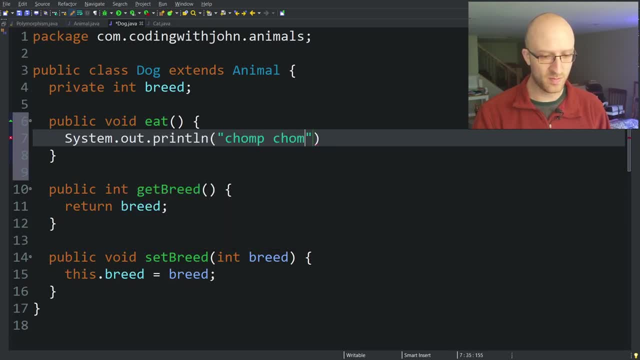 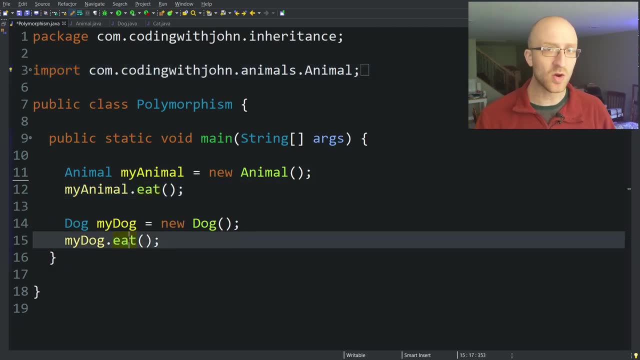 systemoutprintln. Maybe chomp, chomp. We can save that and go back to our main method where we have a regular animal eating and a dog eating. But now this dog will eat in a different way than the generic animal eats. Let's run our program and see what that looks like. Our animal says munch. 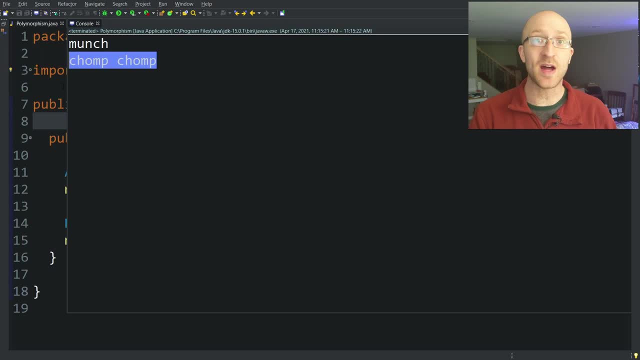 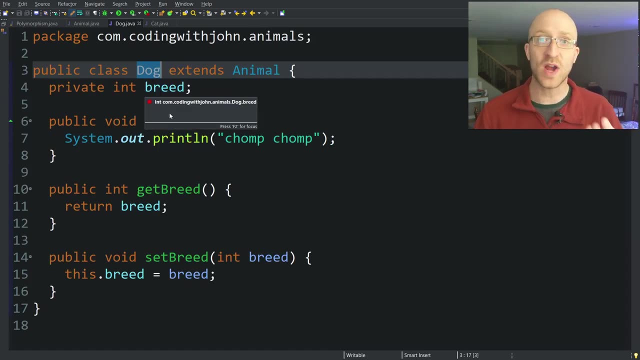 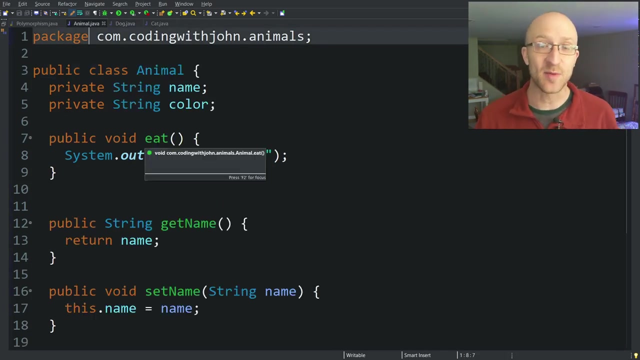 but our dog says chomp, chomp At its core. that's what polymorphism is in the Java world. It's when a child class, like our eat method in our dog class, overrides a method in its parent class. Our dog class's eat method is overriding the functionality of the eat method in the animal. 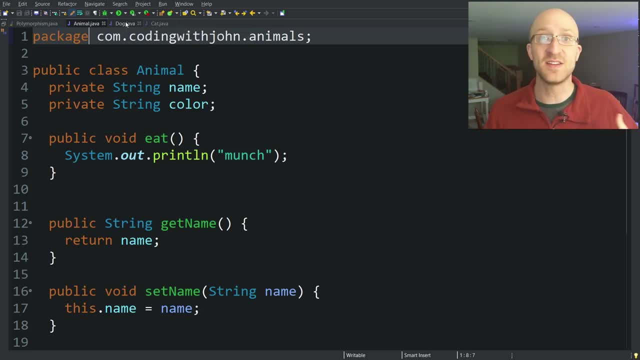 class And because of that we're now doing the same thing in a different form. So that's polymorphism. Our dog class eats in a different way than the animal does. Our animal class gives us certain default functionality for eating, but our dog child class overrides that functionality. 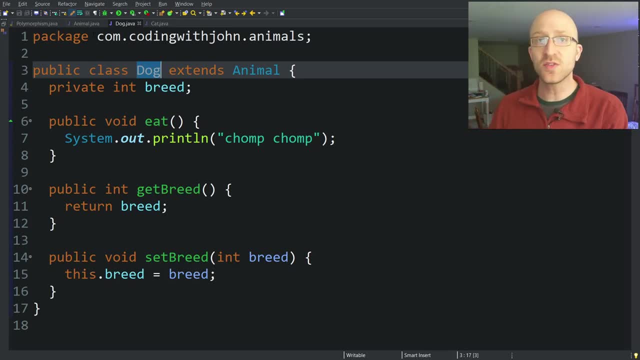 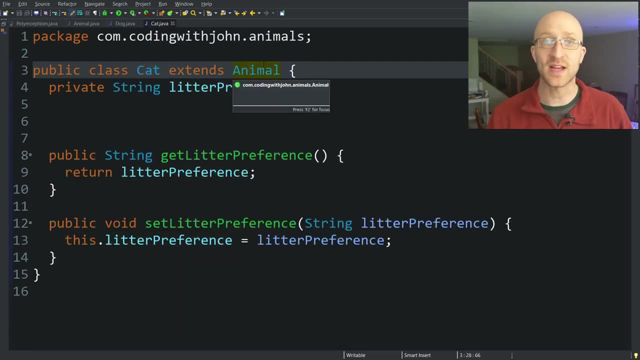 and does the same thing in a different way, And you can have other subclasses that do the same thing, that do the exact same thing. So I've also got this cat class that also extends animal. It's a child of the animal class. also Back in our main method. we can create a cat. My cat equals new. 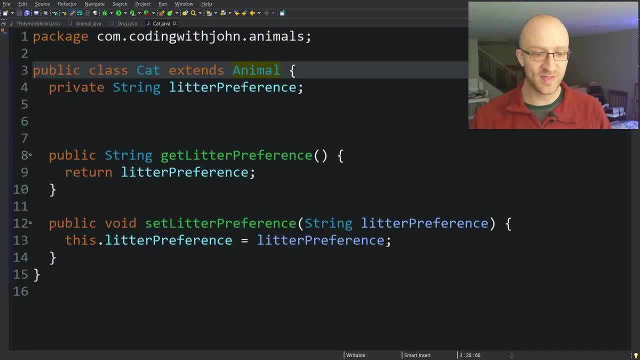 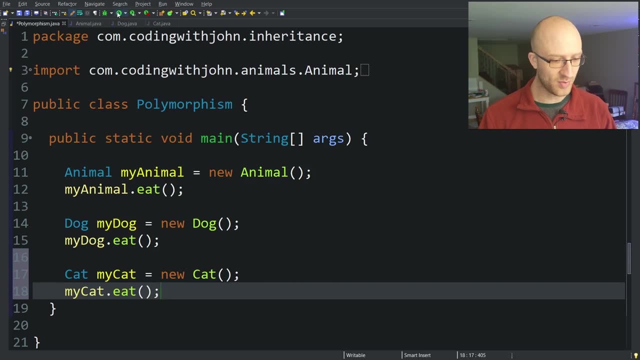 cat And even though in our cat class we don't yet implement that eat method because we're a child of animal, we have it available. My cat dot eat And again we can run our program. And now our basic animal says munch, Our dog says chomp, chomp. because we overrode the eat method from the 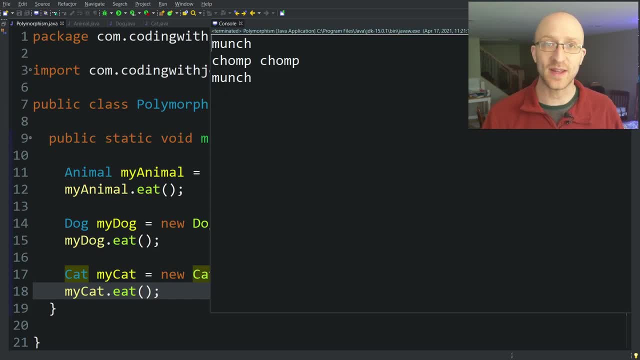 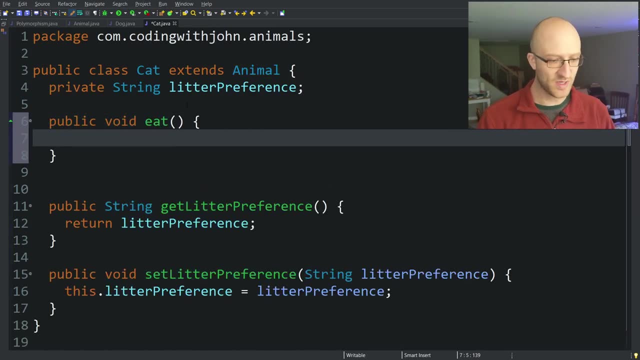 cat. But when the cat eats it also just says munch, because it's not overriding that eat method yet. But we can do that same thing in our cat class Public void eat. And instead of munch or chomp chomp we can say: system dot out, dot print line, nom, nom, nom. Save that. Go back to our main. 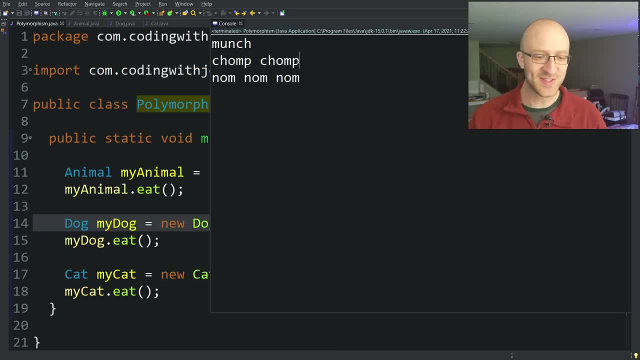 method and run our program again. And now our animal says munch, Our dog says chomp, chomp And our cat says nom, nom, nom. This is just more polymorphism. We're doing the same thing in three different ways, Many forms. We have our parent animal class. 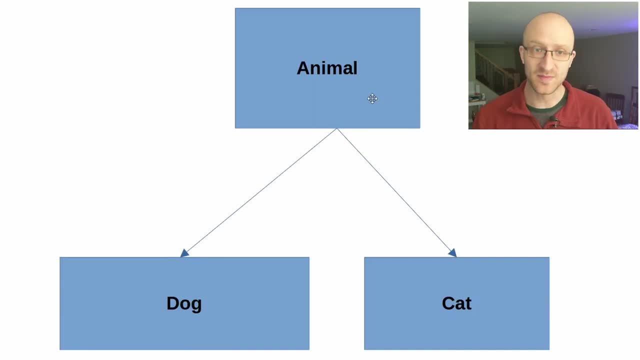 have our dog and cat classes that are both child classes of animal, And all of these classes implement that eat method, but they do it in a different way. Same thing in many forms: polymorphism. Now there is one other form of polymorphism in Java and that's called method. 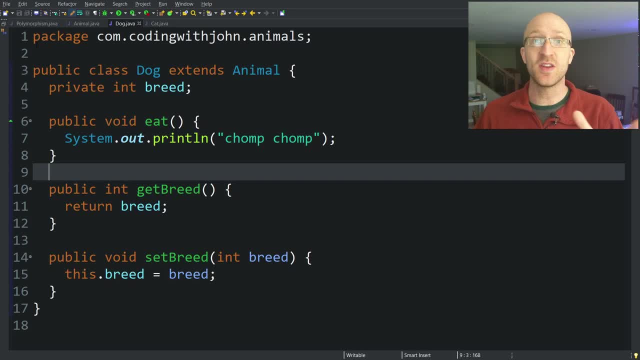 overloading. Now it's really easy to confuse method overloading with method overriding. Method overriding is what we already talked about, where you have a child class that implements the exact same method signature as a method in the parent class. But you can also do what's. 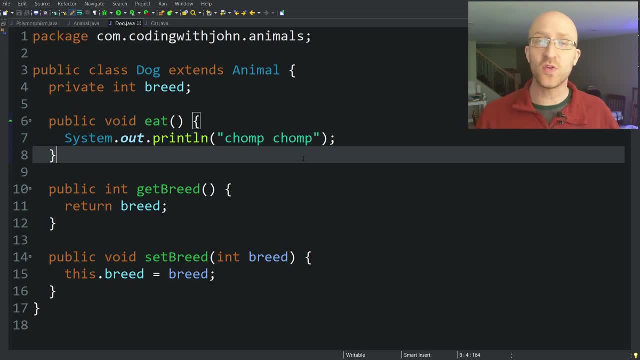 called method overloading. To put it very simply, all that method overloading is is when you have two methods in a class that have exactly the same name but take different parameters. For example, here we have a public void eat method that takes no parameters. Now, of course, Java won't let us.